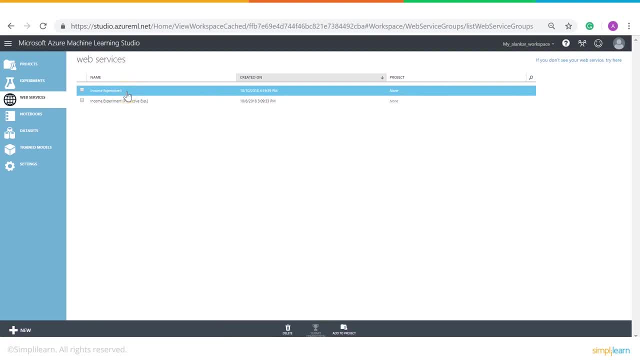 So web services gives you a list of all the experiments that we have and is over the cloud so that you can access it from anywhere. Then comes notebooks. So notebooks are basically space where you can explore analytics. You can create your own code, you can visualize it and, at the last, you can share it with your peers. 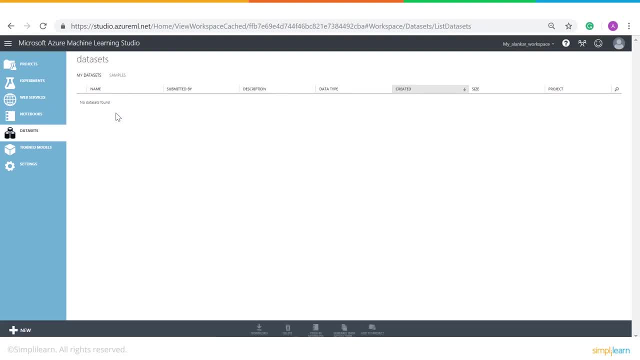 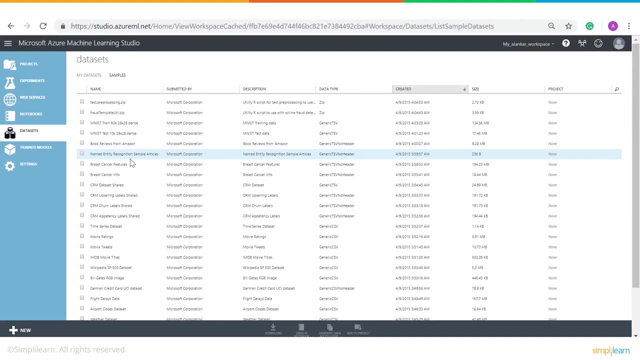 Then is data sets. So the data set gives you a list of all the data set that you have in your Azure portal. Now, when you click on samples, these are all the sample data set that Azure has provided as to the users. Now comes train models. 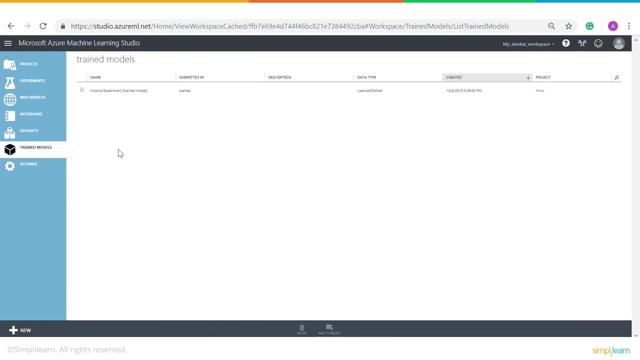 So, while working in an experiment, you will come to a point where you need to train your model. So this gives you a list of all the models that you have trained in your Azure program. Then, at the last, you have settings. So any changes that you make is done under settings. 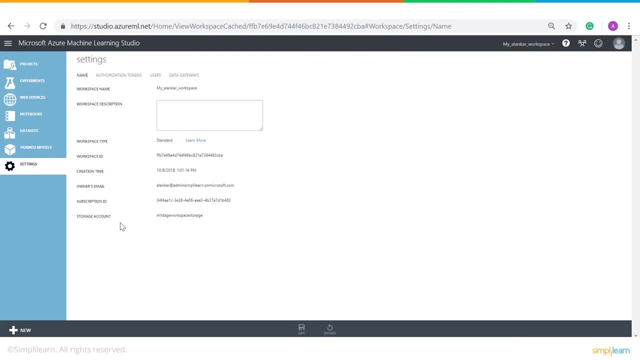 So now that we are done with this, let's go to the next half of our Azure tutorial. So on the left hand side you can see there's an option called new. So when you click on new it will open a window. 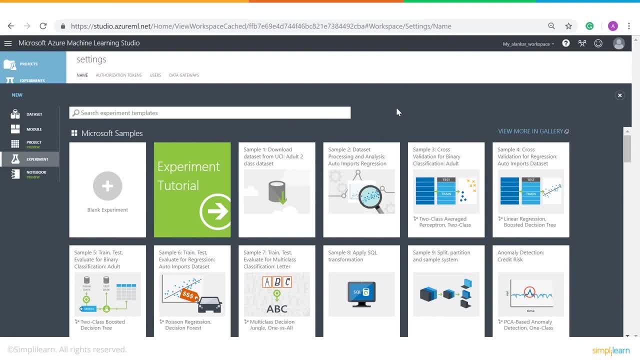 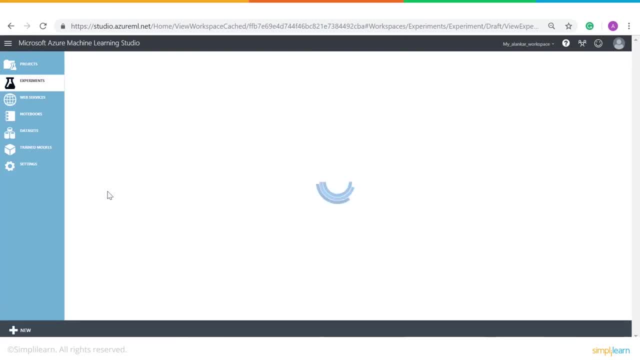 So this window gives you a list of all the templates that we have in our Azure machine learning studio. So since we are working from the start, we'll be working on blank experiment. So once you click on blank experiment, a new window appears. 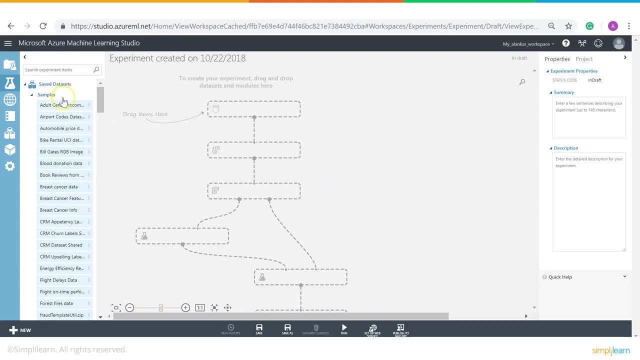 OK, so let me go to the conference that we have here. So on the left hand side you have the components, At the center you have the canvas where your experiments will take place, And on the right hand side you have properties. 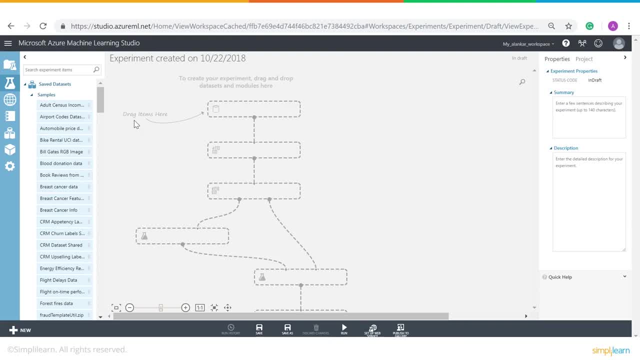 So today we'll be working on problem statement, which says that we need to find the problem statement, So we need to find out the income of an individual whose data we don't have in our system. Now let's go on to the component part and find the best data set that can suit our problem statement. 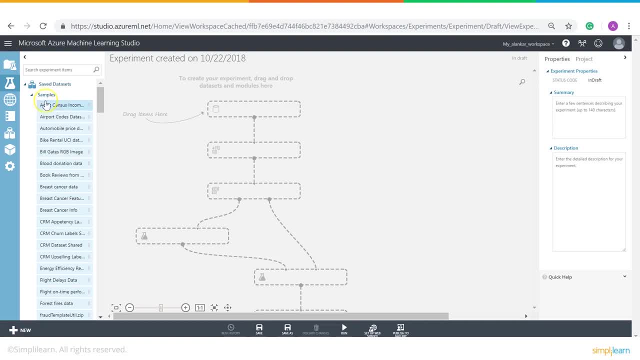 OK, so we see that we have a list of data set in our samples. So the very first data set in Adults Sense is income binary classification. So we'll select the data set and drag it over to the canvas. But before that let me give a name to our experiment. 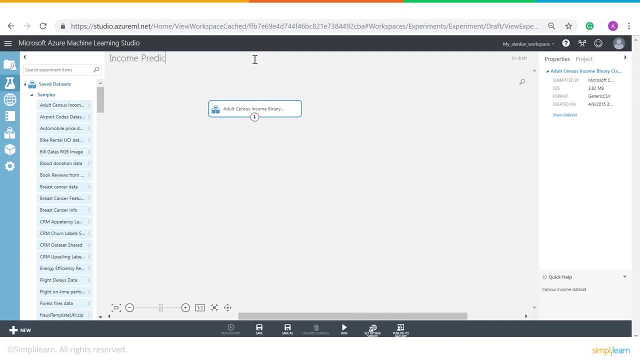 So we'll give the name as income prediction. So we'll give the name as income prediction. So we'll give the name as income prediction. Now, once you click on Adults Sense's income, you can see there is a circle. Press right click and four options appears in front of you. 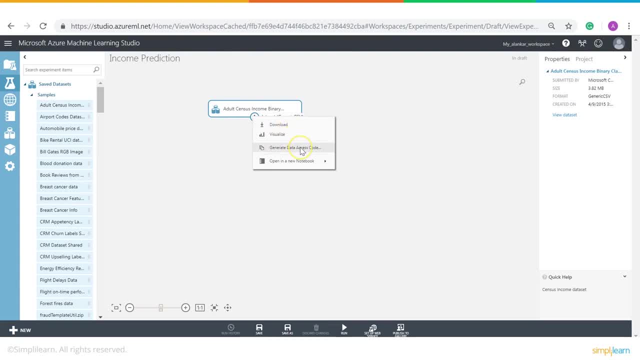 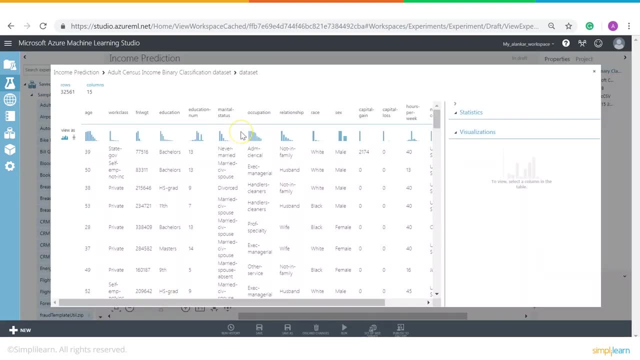 The first one is download, The second is visualize, Third is generate access code And the last one is notebook. Since we need to visualize the data set, we'll click on visualize. So once you click on visualize, a new window appears. 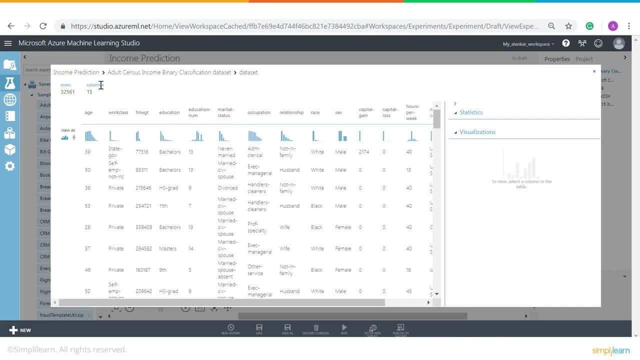 On the left hand side, you can see there are 32,000 rows and 15 columns that we have in our data set. But before that, let me go through all the columns that we have here. So the first one is age, which tells you about the age of a person. 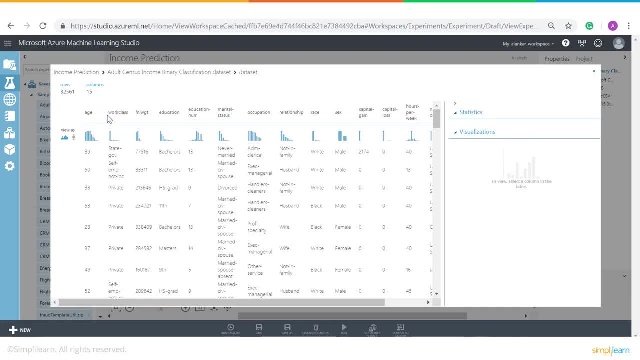 Then is work class. So this gives you an idea whether he's a government employee, is he working in a private sector or is he a self-employed. Then is FNLWGT, which is the sample weight of the field. Then is the education. 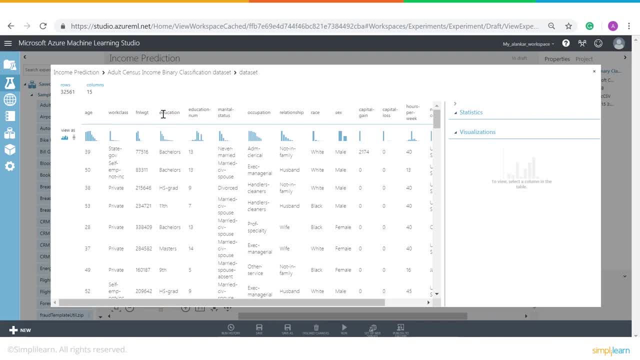 So education is basically telling us about his highest degree, whether is it bachelor's, is it high school grad or is he a master's. Then comes education number. So this gives you an idea of the number of years he took to complete his education. 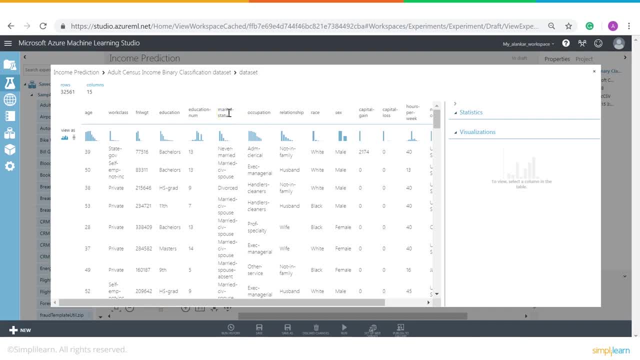 Then is marital status. So this is telling about a person's- is he married or whether he has never married. Then is occupation. So occupation is actually important while finding out the income. So if a person is a manager, there are chances he'll be earning more as compared to others. 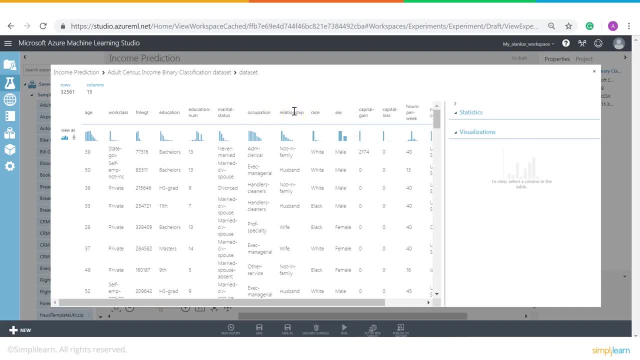 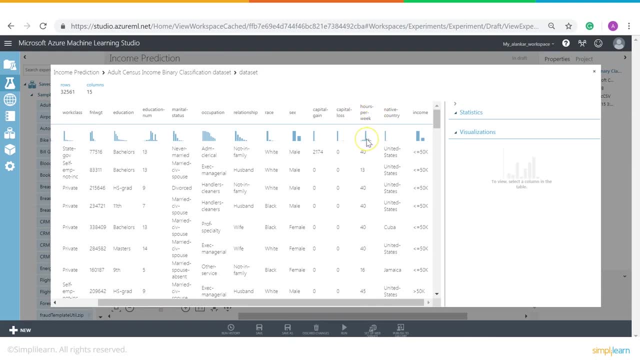 Then is relationship, whether he is a husband, is she a wife or has he never married. Then comes sex, whether he's a male or the female. Then is capital gain, capital loss: hours per week. So this gives you an idea of number of hours a person is working in a week. 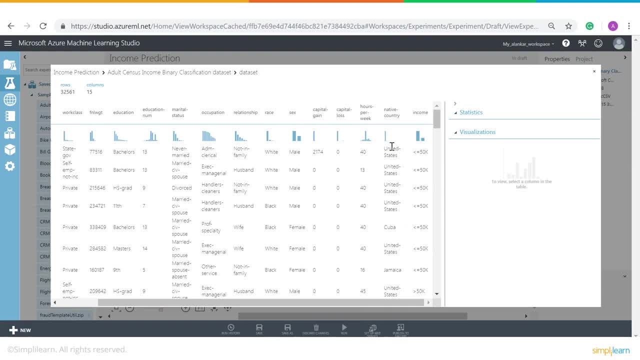 Then is income. So income varies from country to country, So getting to know about the country is also very important while predicting our model. And at the last we have income. We see that the income column is divided into two halves, which is above 50 and below 50. 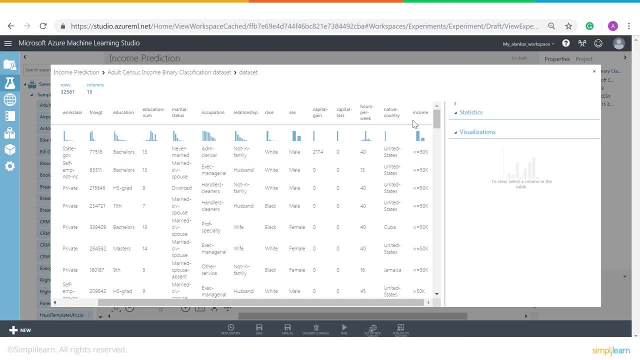 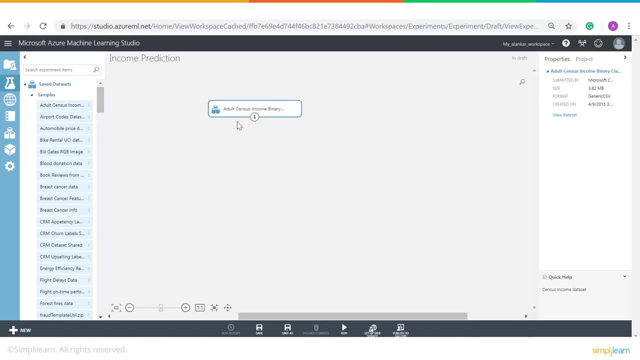 So there are two distinct values in income group, And in cases like these, we make use of classification algorithm. Now let's go to the next part, which is where we will define that field that we need to have for our prediction. So what we do here is we select the column. 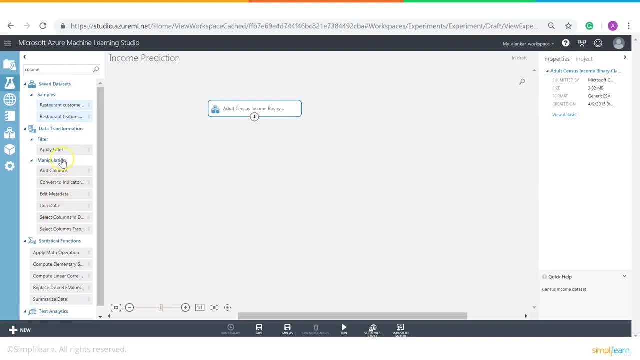 So on the search bar when you type column under manipulation, you get a list of options. From that you select column in dataset and drag it over to the canvas. Now connect your dataset with select column in dataset. Now under this you can see there's a caution which says that value required. 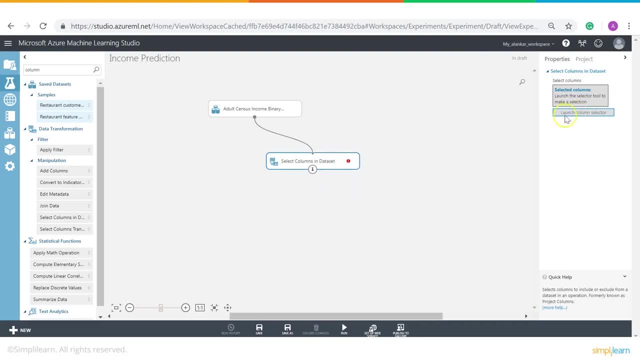 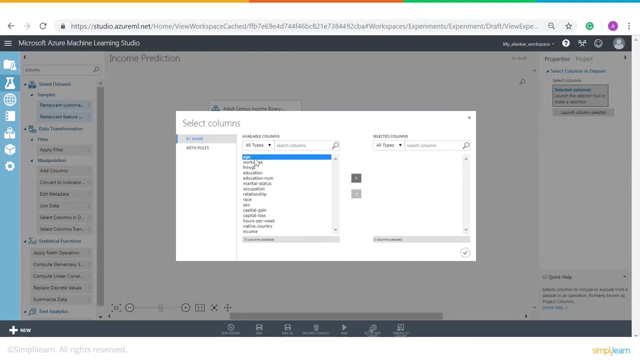 So you go under properties and select launch column selector. So once you select launch column selector, window appears. So this gives you a list of all the columns that we have in a dataset. So the very first column that we have here is age. 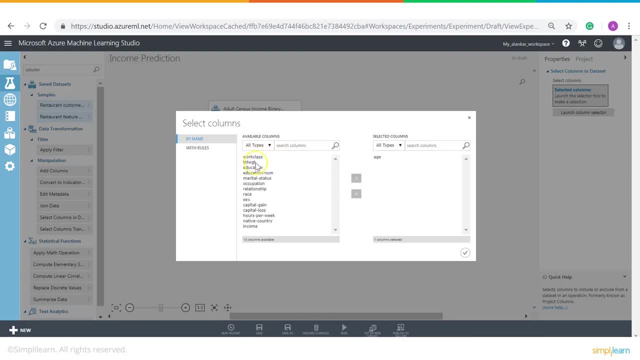 So age is actually important in understanding your data set. So age is actually important in understanding your data set. So age is also important in understanding the income of person. So age is also important in understanding the income of person. then comes work class. 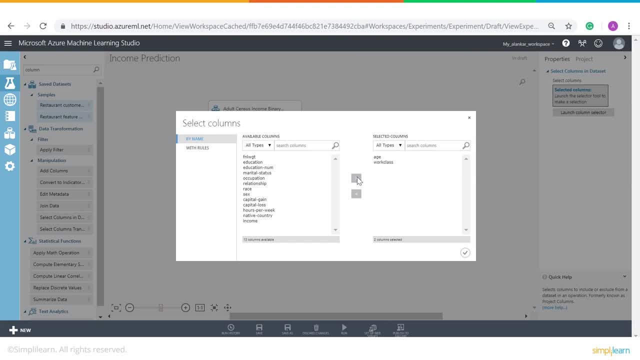 So the background of a person, whether he is working as a government employee or is he a private employee, is also important for prediction of income. Then comes education. A person who has a master degree has more chances of earning than a person who has a. 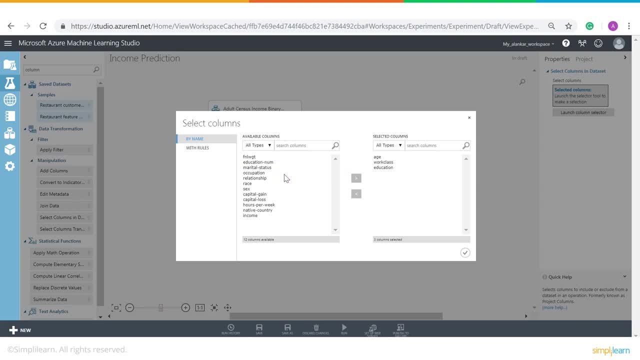 graduate degree. So education is also an important field. when predicting an income, then what comes next is occupation, After that you have country And at the last we will work on income. now, when you press next, you get back to the same window. so now that we know the field that we are, 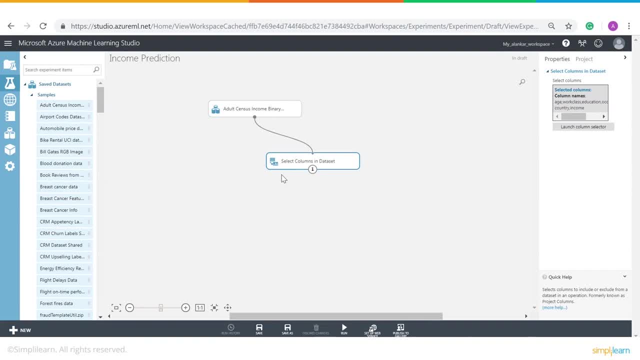 working on. our next step is to find the algorithm that best suits our model. okay, so now that we know the field that we have to work on, our next step is to find the best way algorithm for our model. so what we do here is we look at the list of algorithms with that we have. but before that, 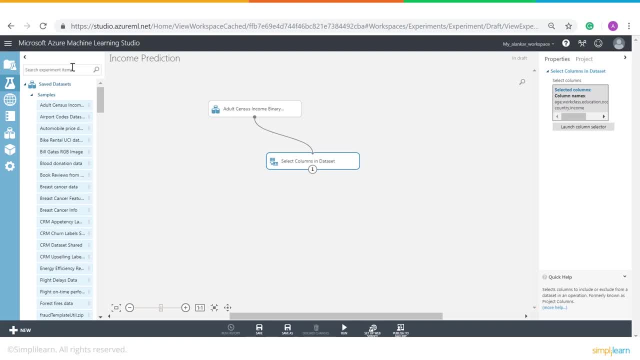 we know that our data, our target value, is divided into two classes, so the algorithm that we'll be working on is a classification algorithm. now, azure provides few classification algorithm, like logistic and decision tree, two class boosted decision tree. so we'll be working on two class boosted decision tree because this gives you a high accuracy rate. now let me give you an idea. 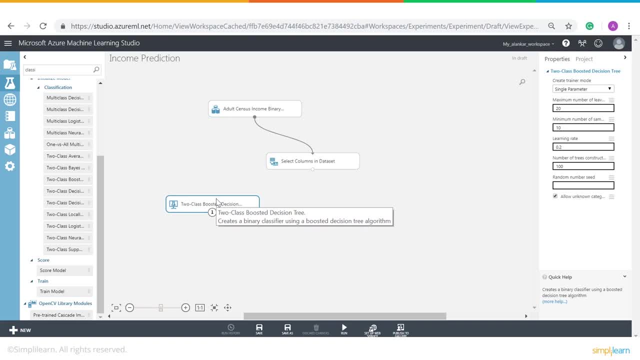 of why two class boosted decision tree is taken over all the other classification algorithm. so what happens in two class boosted decision tree is for every node that we have here the accuracy is calculated, and once the accuracy is about above our required accuracy, then only it moves on to the next nodes. so this gives you a high. so the 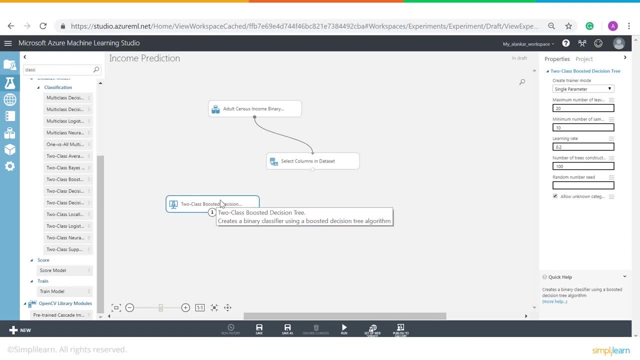 prediction value here becomes more and more towards a higher side, so that the overall model will give us a very high accuracy. okay, so our next step here is to train the model. so on the search bar again, just type train, and under train you can see there's an option called train model. so drag the. 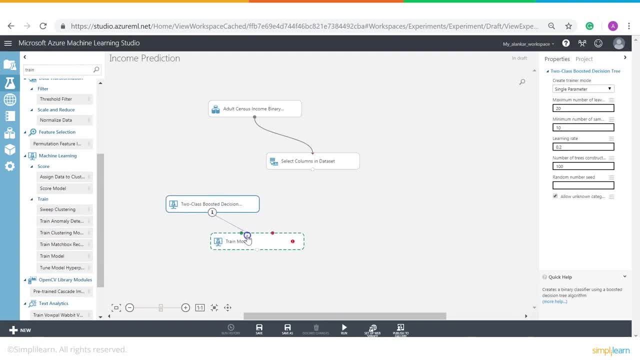 train model over the canvas and connect the two class boosted decision tree with this. now you can see the data in the data tab and it says that it requires a value or a data, which is obvious. because it's not, it does not have any data to work on. so our next step here is to split the data. so, on the search, 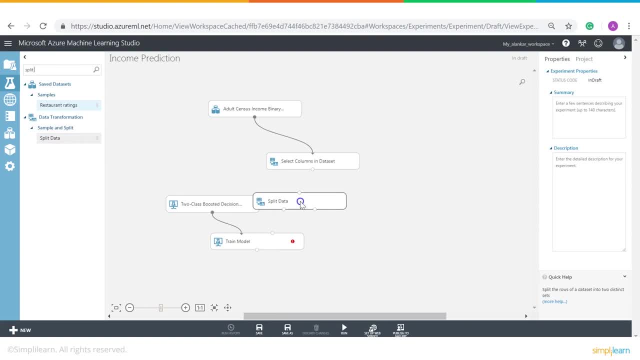 bar. when you find split, it gives you an option called split data. when you drag the split data over the canvas and connect it with your column data, it asks you for the split percentage. so you split the data into training and testing. so eighty percent of data gets into the training model and 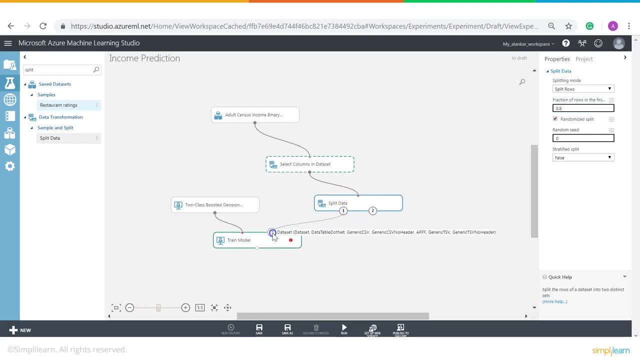 So what we do next is we connect 80% of training data with the trained model. But you see, there is a value required. This is because the model is not aware of the column it needs to train on. So what we do here is we go on launch column selector and select the column. 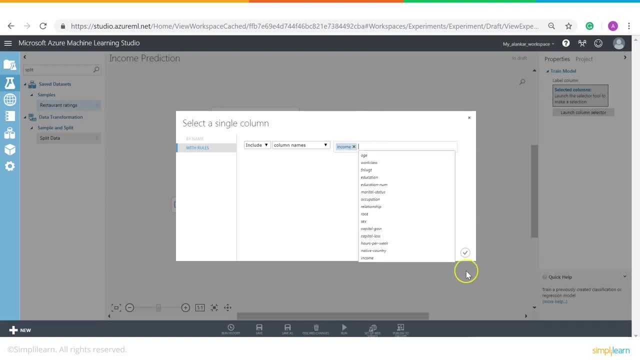 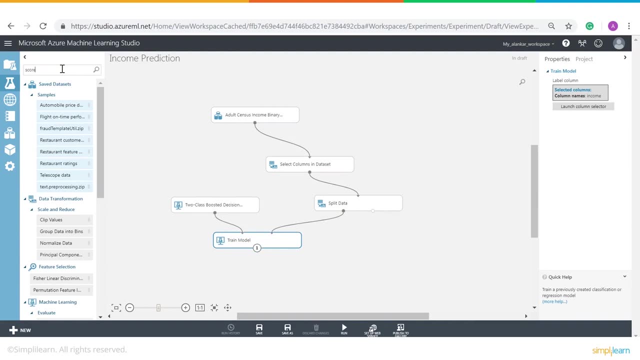 So we need to work on income column. So when we select column and press enter, we see that the question mark is gone. Now our next step is to find the score of the model. So what score does is? it gives you the prediction value of the model. 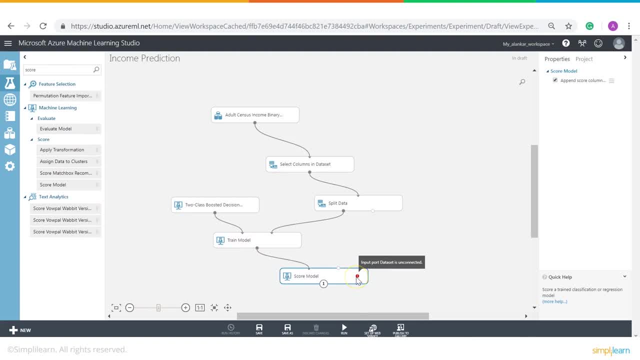 Okay. so when you connect your trained model with the score model, you again see a caution sign here. This is because it does not have idea of what it needs to test on. So you connect your testing data with your score model. So our last step here is to evaluate the model. 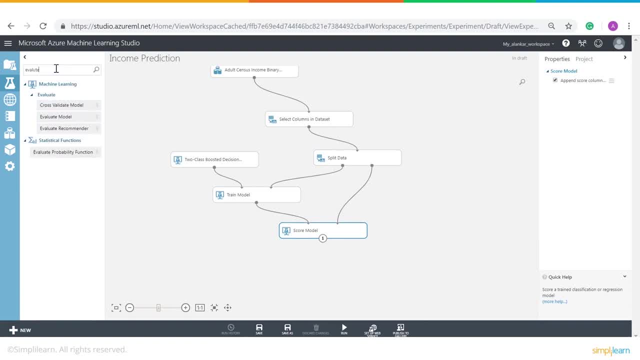 So on the search bar, when you type evaluate, you get an option called evaluate model. You drag the model here on the canvas and connect it. So your model is now complete. Now our next step is to save the model and run it. 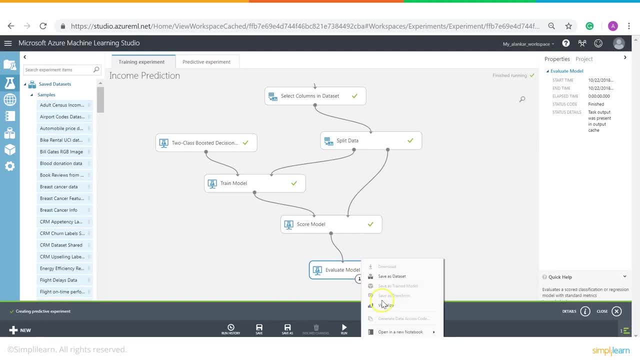 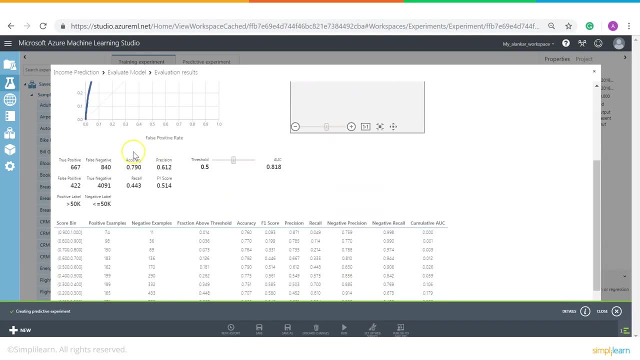 Now, once our program is executed, click on evaluate model. Once you click on evaluate model and press visualize, a window will appear. This shows you the performance of the model. You see that the accuracy is 79,, which is considered to be good. 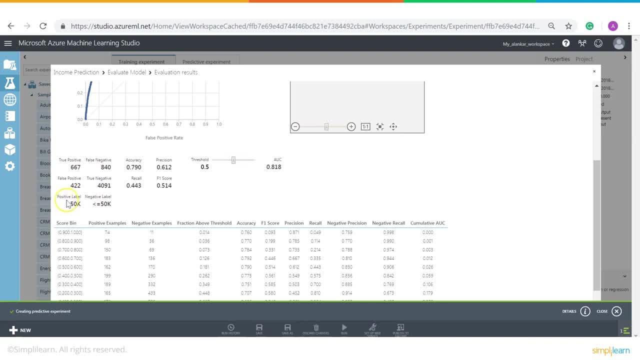 Now let me go through all the other options. You see, there is an option called positive label and negative label, which has been assigned values of above 50k and below 50k respectively. Now let me tell you what these values are. 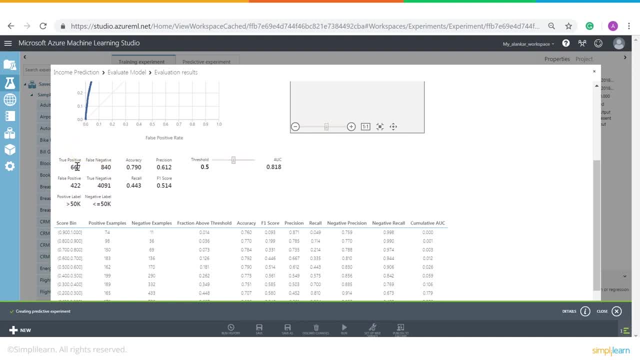 So this part is known as a confusion matrix. So of all the values above 50k, true positive give me value that are predicted correctly, and false positive give me value that are not predicted correctly. which means that out of all the value that we have in positive label, 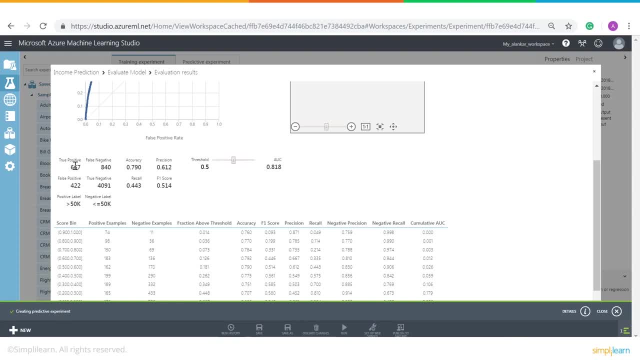 6, 67 have been predicted right, That is, they have their salary above 50k, and 422 have been predicted wrong. Similarly, they are out of all the people that we have, 840 have been predicted wrongly, That is, they have salary of above 50k but have been predicted below 50k. 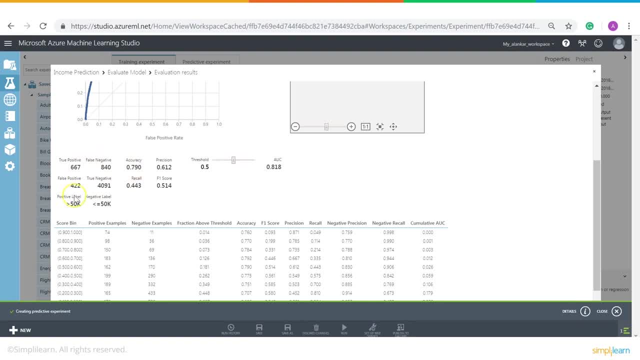 And 4091 have been predicted correctly. Now this is used to find the accuracy of the model. So what you do here is you sum the true positive with true negative and divide it by false positive, false negative, true positive and true negative. 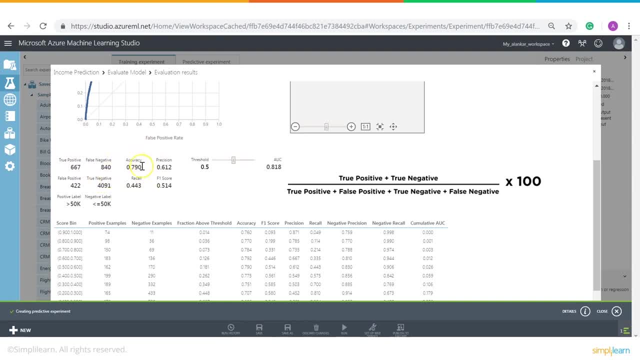 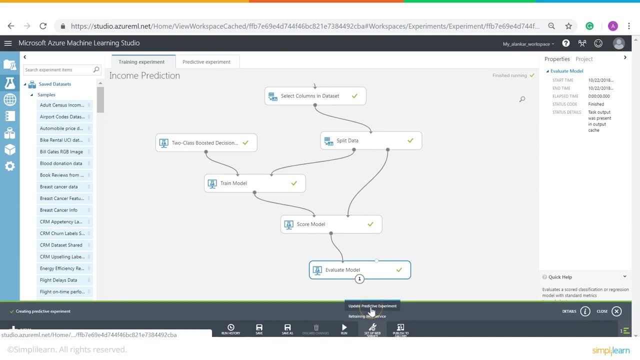 And then you multiply it by 100. And that's how you get your accuracy. Now let us go back and run this service over the net. So when you click on set a web service, you see predictive experiments. Click on predictive experiment. 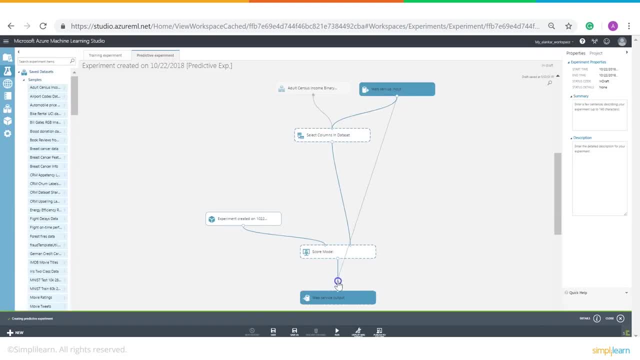 Now our next step is to connect the web service input- that is, the entry point- with the score model. So what it does is, once the program is over the cloud, it directly connects to the score model and shows us the output. So you don't have to go through all the processes. 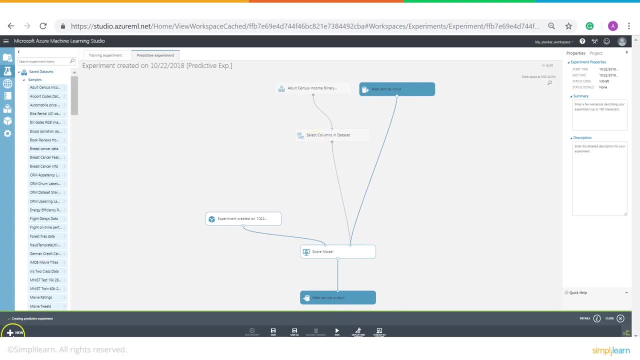 Now, because the machine is automatically learning. Now you save this and press run. This will execute the entire model. So once this is done, all that is left with you is to deploy a web service. So once you click on deploy web service, it will take you to the dashboard. 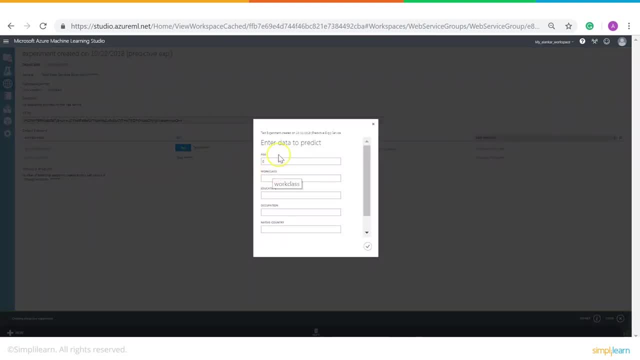 So you see an option called test. Once you click on test, it will take you to a window where it will ask you for values. So let's just say that I have a value of person age 35.. Let's say he's working in a government. 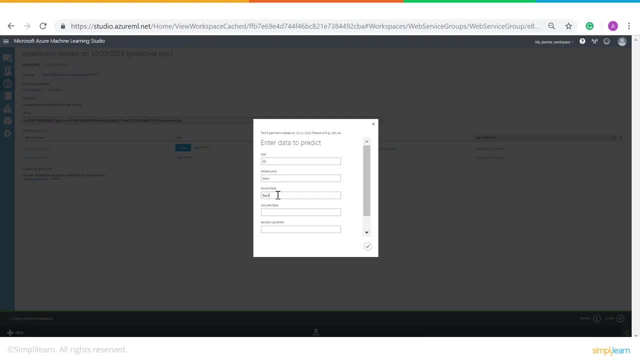 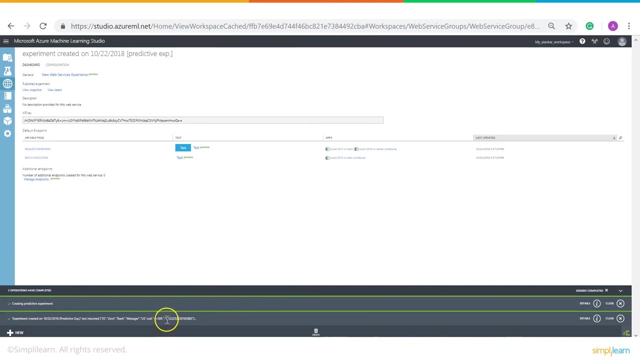 His education is bachelors, Then his occupation is manager. His country is US, So once I press next, it will give me the predicted value, telling me that he will be earning 50k with a precision rate of 0.12.. 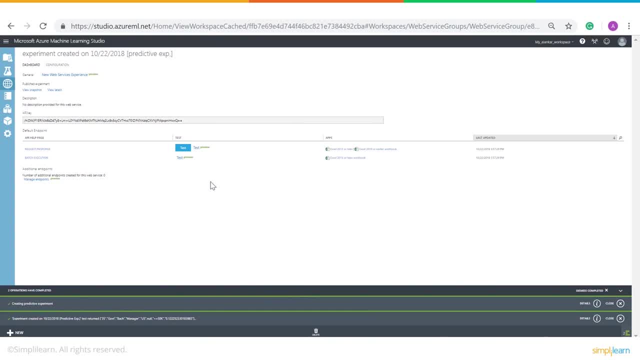 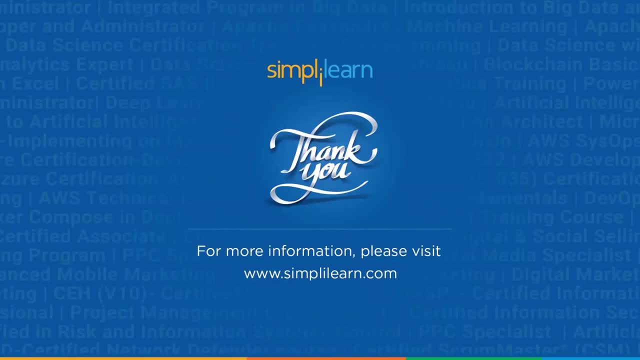 So this is how you make use of machine learning in Azure. So with this we have reached the end of the video. I hope you found it helpful and informative. Stay tuned for more such videos from Simply Learn. Thanks for watching. 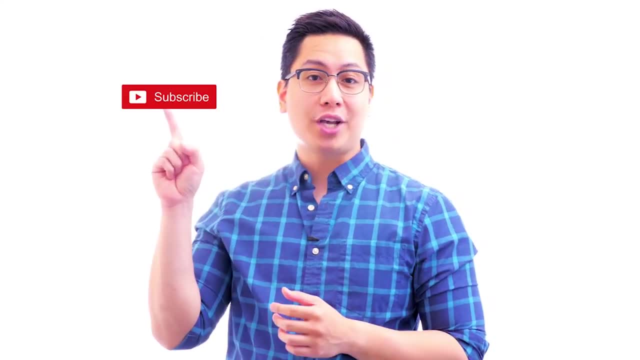 Hi there. If you like this video, subscribe to the Simply Learn YouTube channel and click here to watch similar videos. To nerd up and get certified: click here.